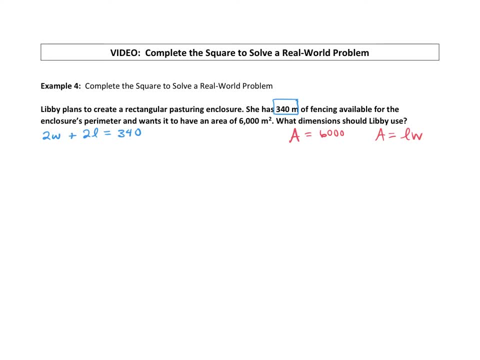 So I'm just going to go ahead and solve for the width. To get that W alone in this equation over here, I'm going to subtract 2L from both sides. That leaves us with: 2W is equal to 3.5.. 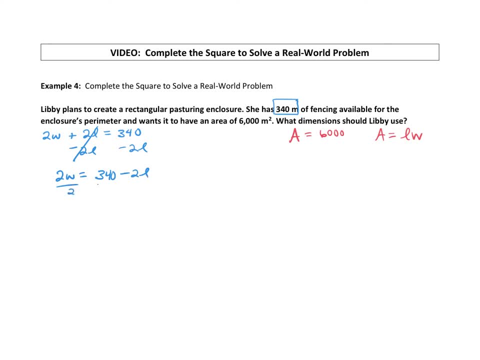 340 minus 2L. Let's divide everything by 2 so that we can get: our width is equal to 340, divided by 2 is 170.. And then 2L divided by 2 would leave us with just L. so minus L. So our width. 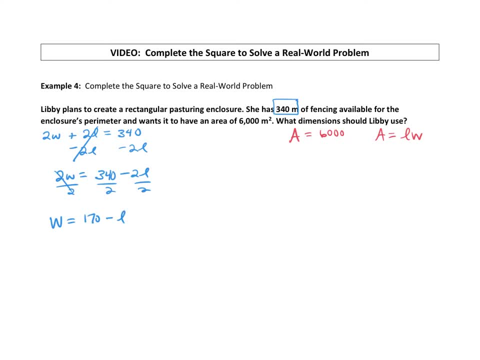 is equal to 170 minus the length, And then our length will still just be the length. So if we come over here to the right, our area equals 6,000.. Let's plug in: Area is length times width equal to 6,000.. We know that the length is L and the width we just said we defined as 170. 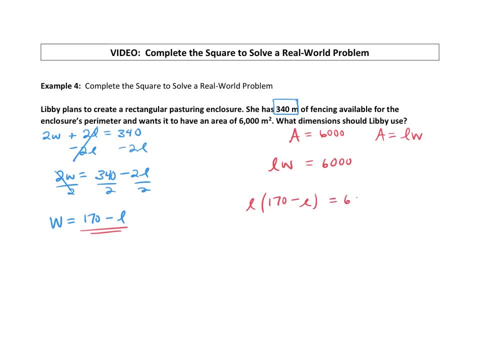 minus L equals 6,000.. So let's go ahead and multiply this out. We now have an equation with all L's, So we're going to be able to find the length that we need, And once we know the length, we're able to get the width, because we'll just take 170. 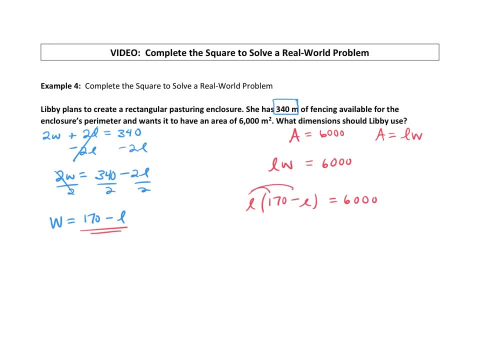 minus the length. So to solve this equation, we're going to go ahead and distribute. This gives us 170L minus L, squared equals 6,000.. Let's write this in the proper order. We know that we want that squared term first, So just. 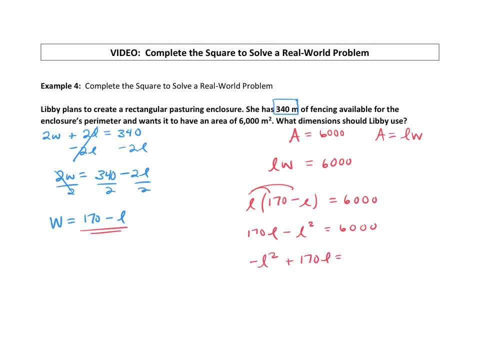 negative L squared plus 170L equals 6,000.. And now let's use that method of completing this equation. So we're going to go ahead and multiply this out And once we know the length, the square, The one thing for completing the square is you do want your squared term to be. 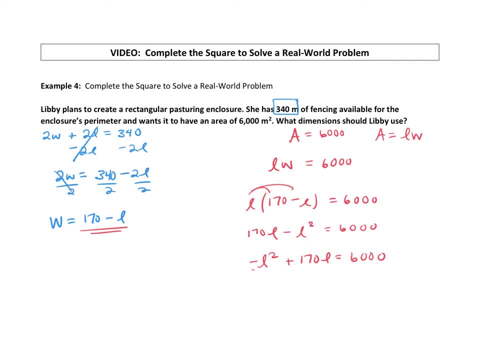 positive. So what we can do here is we can just divide both sides of the equation by a negative one. Basically, every single term divides by negative one. We also could multiply every single term by a negative one and get the same result. That's going to leave us with a positive. 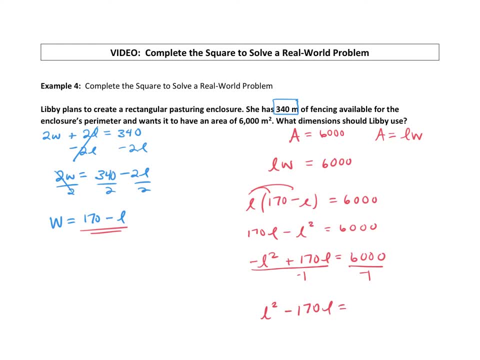 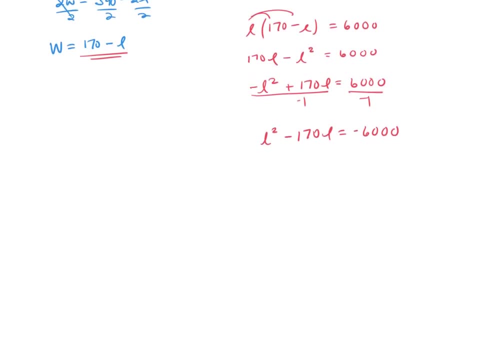 L squared, a negative 170L and a negative 6,000.. All right, our solving method is completing the square. We want to complete this into a perfect square trinomial. So we have to add in what should be our third term so that it's a perfect square. So I'm going to go ahead. 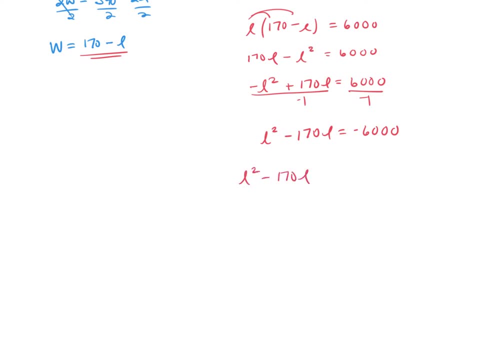 and L squared minus 170L, plus something I'm pushing off, that equals negative 6,000.. So we have a way to get this square to be a perfect square. So we're going to go ahead and add in this third term that we saw in our other videos. If you take your B value, which is negative, 170,. 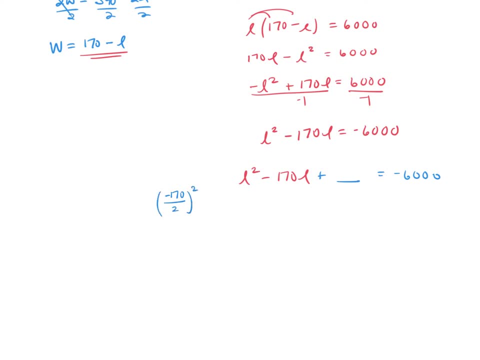 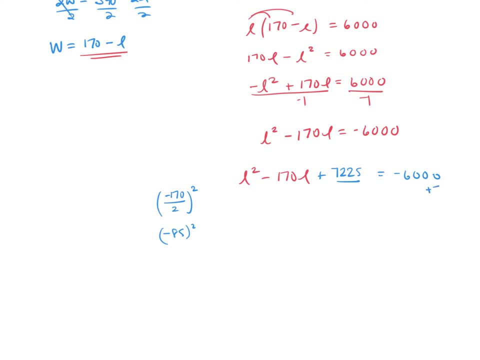 we have to add it in to the other side as well. Okay, this is not probably not super recognizable as a perfect square trinomial, but it is Something. times itself equals 7,225.. And it adds up to negative 170.. You could find that number a couple ways If you took the square. 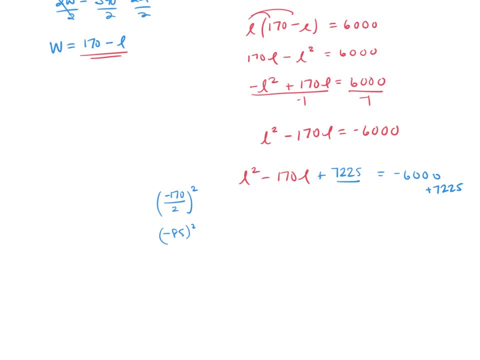 root of that 7,225, you would get 85. So 85 times 85 multiplies to this 85 plus 85 multiplies to a positive 170.. So what if we use two negative 85s? The other thing you may have been noticing is when we do our b. 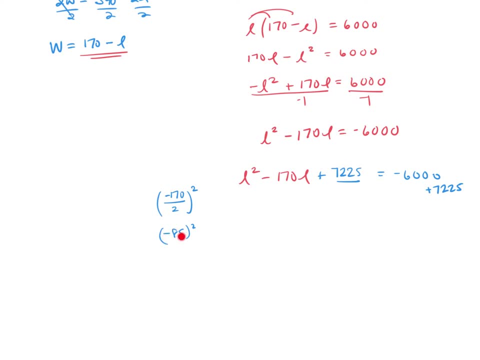 over 2 and then we square it. whatever that b over 2 value was is always what we're looking for to put right into our factored form of this: x minus 85 squared, So negative 85 times negative 85 is 7,225.. Negative 85 plus negative 85 is a negative. 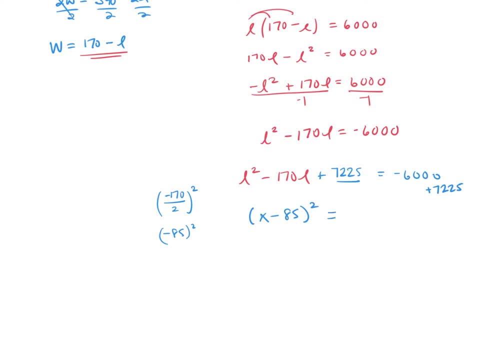 170.. Okay, so that is equal to. when we combine these terms over here we get 1,225.. Okay, now we're going to solve for x. Oops, not x. Did you guys catch that? That should be. 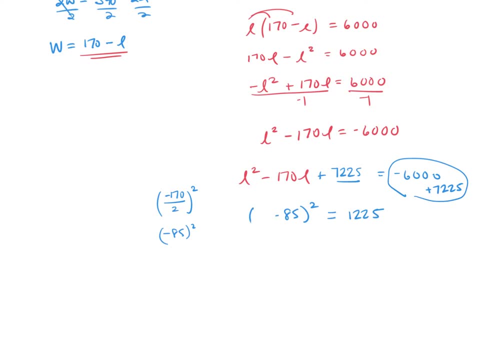 an l. Let's see if it will. even let me erase it. Oh, there we go. I'm so used to using l's. There we go, l minus. So let's square root both sides. When we square root, we cancel. 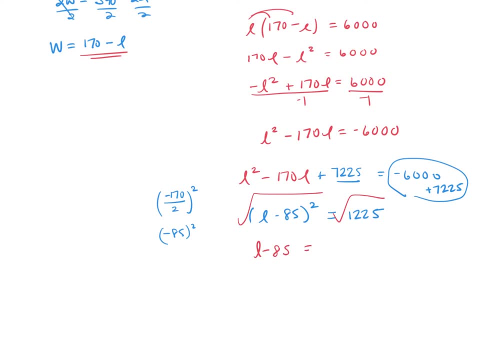 the square, leaving us with l minus 85, equals now the square root of 225, 1,225.. We get two answers when we square root when solving these equations, And then this is a perfect square: Square root of 1,225 is 35.. 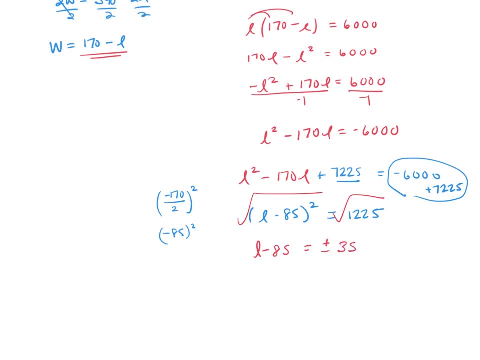 So we're going to use the square root of 1,225.. So we're going to use the square root of 1,225.. So here's where we're going to break it into our two equations: l minus 85 equals 35.. 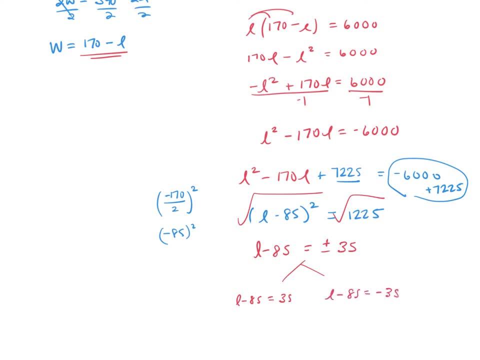 And l minus 85 equals negative 35.. So we're just taking this positive and negative 35 and splitting it up into our two equations. If you add 85 to both sides on this one, we get 120.. If you add 85 to both sides in our second equation, we get a positive 50.. 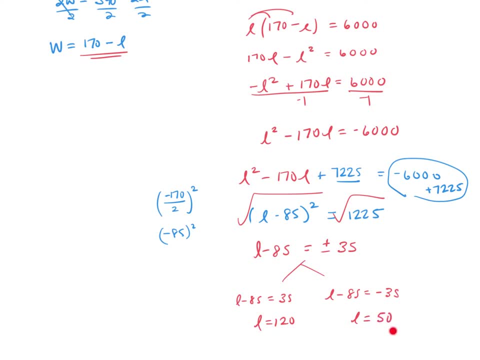 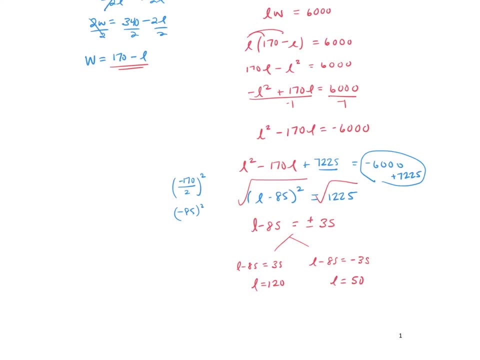 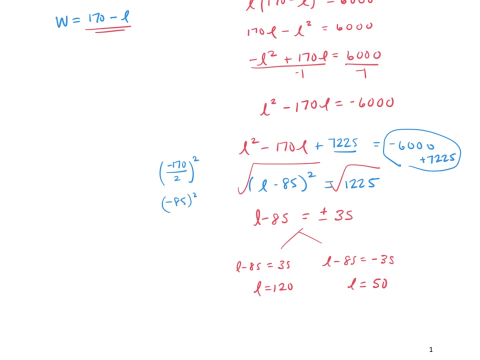 So we're finding that the length can be 120, or the length could be 50. Those are both plausible answers, so how do we know which one it should be? Well, let's see what we think about that If we plug those in. so let's try to change my marker color. Here we go.